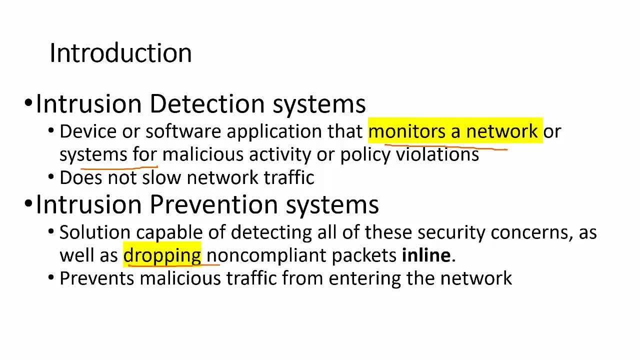 it will drop the packet. That is why we call IDS used to detect the intrusion, and IPS used to prevent the intrusion. So intrusion is basically mean any action which is attended by the attacker to compromise the network or anything which is accessing in an unauthorized manner. That is called as an intrusion, like uninvited guest. 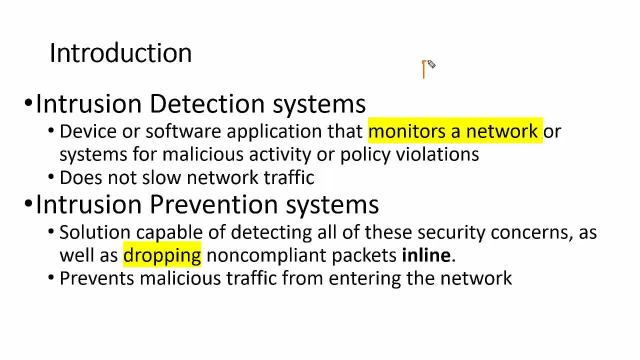 So example like this is my IDS, we have, example, intrusion detection system, Okay, And we have a user one, And this is my web server, Okay, so user sending a traffic. Now IDS will basically capture this traffic and compare against the rules, which is basically create. I'm just 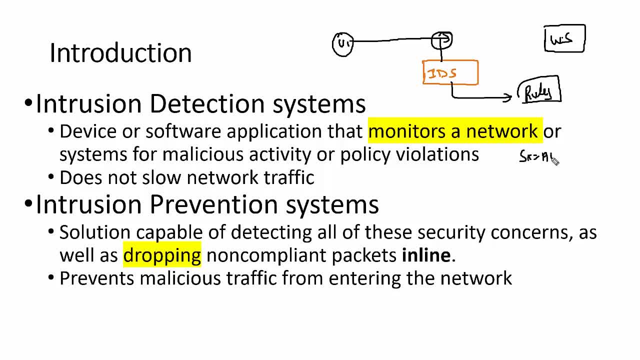 taking example, by defining a rule here Is: source is any, destination is basically a web server. source port is any and destination port is 80. So what happened is we have created this rule, which defined as a legitimate traffic behavior. Now IDS will capture the traffic and check the context of the traffic against. 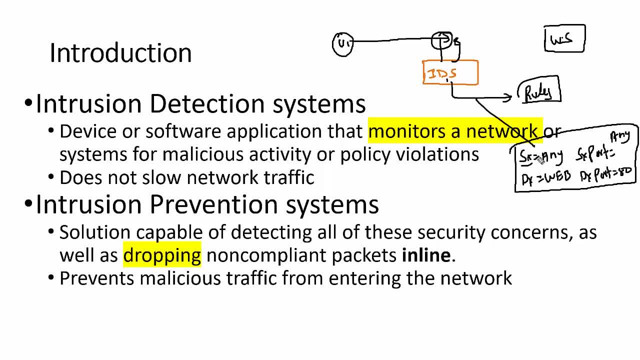 this particular rule we have: yes, source is any. we cannot, we cannot, we can ignore that destination. this packet is going on a web server. source port is any okay, but destination port is not a 80 in the packet. it's showing me 27 or 23. so ideas will basically log that. 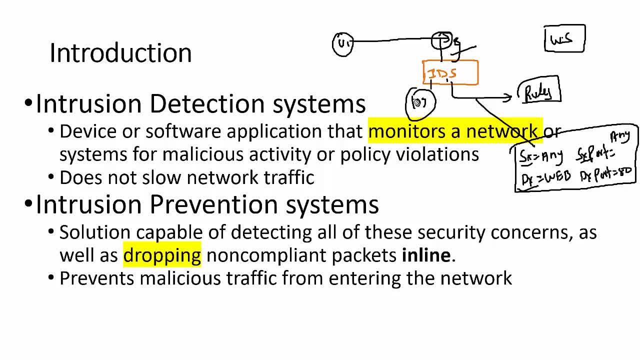 traffic okay. so that is a role of ideas. but if I say we have a IPS, in that case it will basically block that traffic. it will drop the traffic. that is why ideas is also called as a outline mode and IPS is called as a inline mode. it mean if 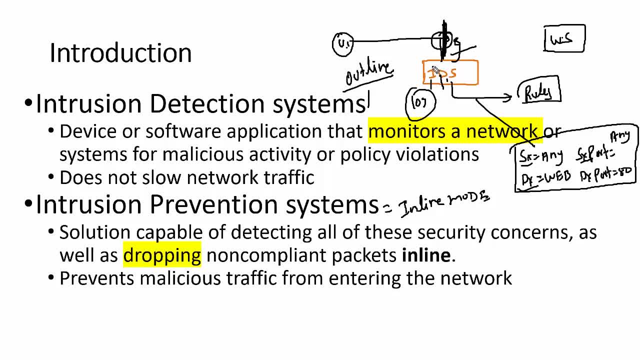 user sending any traffic to web server. if the traffic doesn't meet. as for the IPS, it will block there itself. it will not reach the web server, but in the ideas it will remain outline, it remain passive and just have a allow the traffic to be go on a web server, but it will lock the traffic. that is why 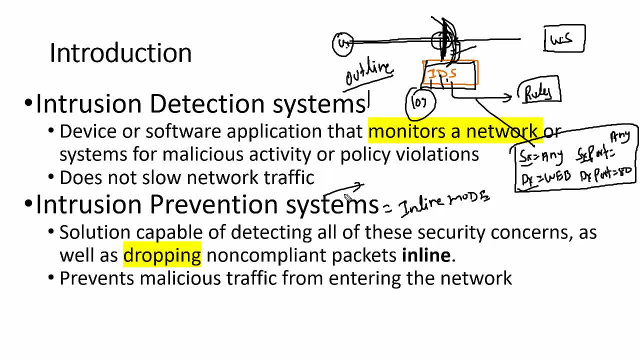 I PS load on the performance where the IPS- sorry, IPS- will basically slow down the performance with the ideas will not slow down the performance. that's why it's clearly mentioned in ideas does not slow the network traffic because it will not block. but in the case of IPS it will basically block. that's why it will. 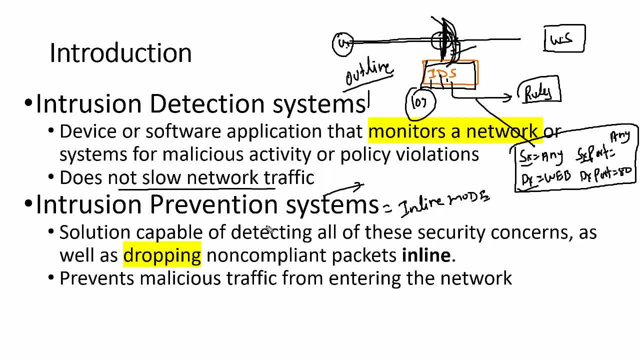 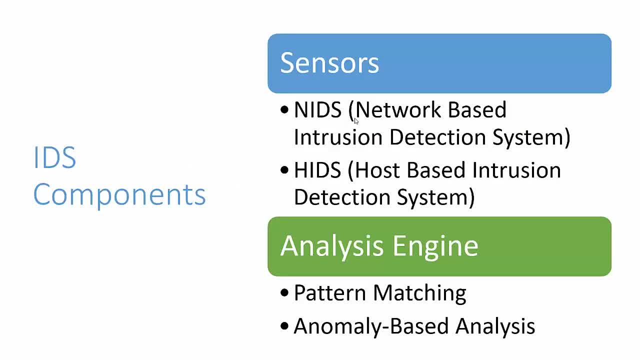 impact the network traffic, but ultimate goal of IPS and ideas is different. so that is a thing we have now when you're talking about ideas component, because we need to include a feature like a sensor in the process, so let's talk about it, okay, so what we have first here is a sensor we are specifically talking about. 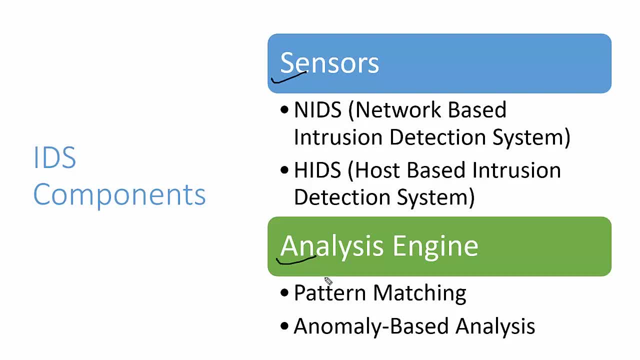 in this session, ideas. so ideas basically has a two component: one is called as a sensor and one is basically called as an analysis engine. ok, so first we discuss about the sensor. so sensor is to type network based intrusion detection system and host based intrusion detection system. so what is an ID s and what is a? 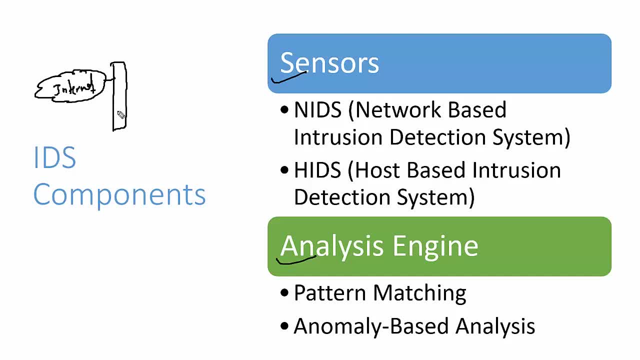 idea. suppose this is my network internet on the border of the network, and then we have a switch here and then we install the system a, we install the system B and we install the system C. okay, so now what happened? the traffic is basically coming from outside, so NIDS will. 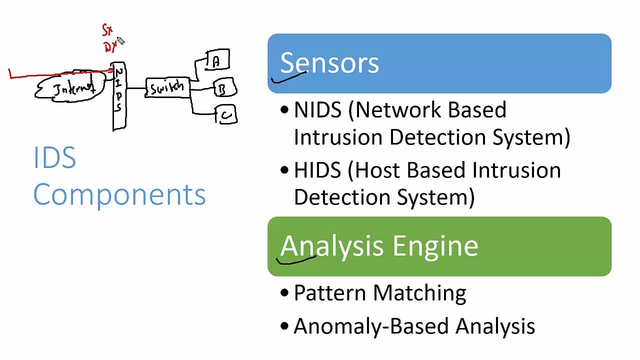 monitor from where it is coming to where it is going. it also monitor from which port is coming to which port is going, but once the traffic is passed to the NIDS, what kind of a changes it introduced in every system that NIDS will not able to monitor. for that we need to install in every system HIDs. 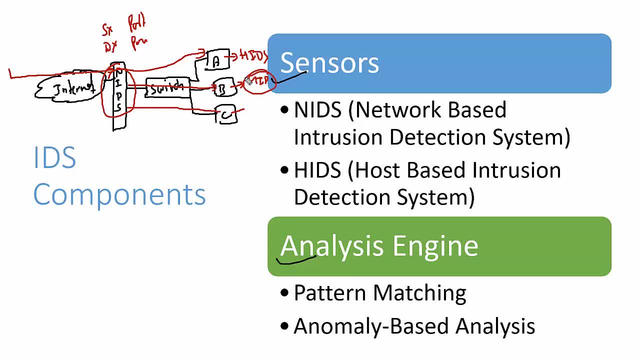 okay, so NIDS is basically used to monitor the network level traffic and HIDs is basically used to monitor the host level traffic like modification attempt in a system level and all that. so we have a tools like tripwire and all that. but one concern with installing HIDs in every system is: 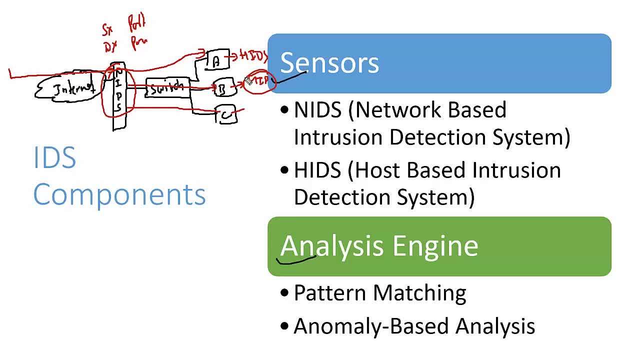 that performance issue. okay, so that is the NIDS and HIDs. so that's why we prefer to install the NIDS in the border of the network, which monitor all the traffic which is coming to the enterprise network. and if you want a system level activity, we install the HIDs in every system, just like our. 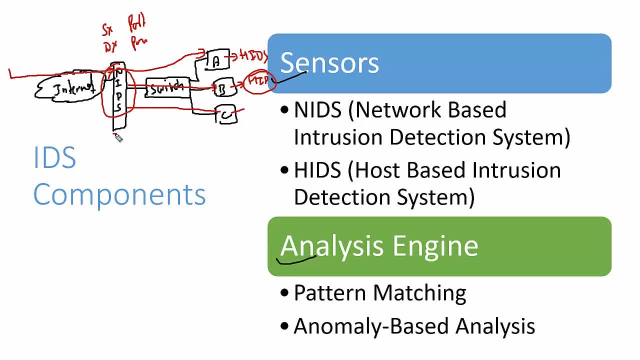 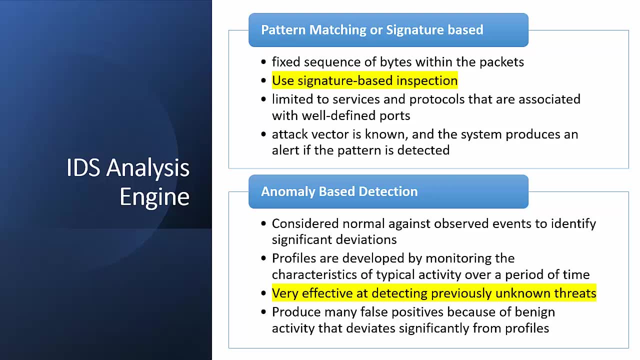 antivirus. but the question is how do we install the HIDs in every system and the question is how they detect the intrusion. so they have a two-way to detect the intrusion, based on a pattern matching and based on anomaly. that I'm going to discuss in my next slide. so we have discussed so far about IDS. 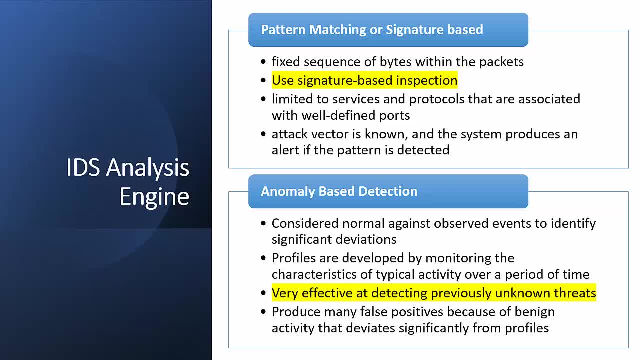 component which is called as HIDs and NIDS, and that is a two type of sensors we have that we place in the border of the network or in a one particular host, and the second part is basically called as an analysis engine. but the question is, you know based on what factor it able to detect the intrusion? so we have a two. 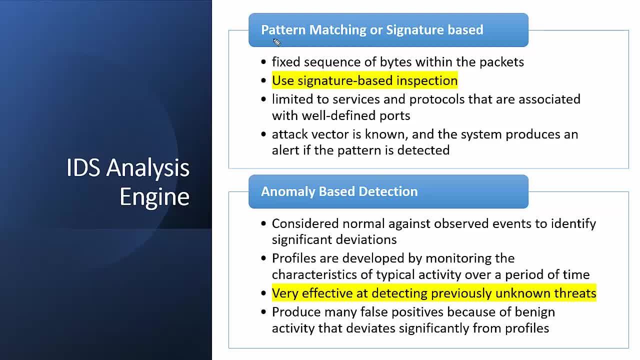 type of intrusion detection mechanism we are using. one is called as a pattern matching, which is also called as a signature based intrusion detection, and second is anomaly based detection. like example, we have an antivirus, the antivirus that we installed in a system. it basically scan the file, check for the 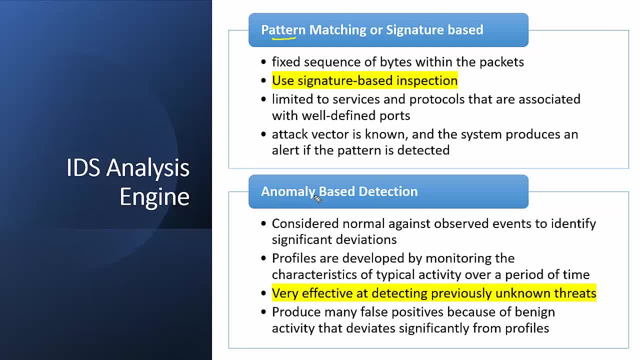 signature and compare against the database signature match. they will give alert, it will block. so same, like IDS and IPS use sensors, they use a- sorry, they use analysis engine. they use this mechanism based on which they detect the intrusion. so first, which is a traditional method, is called as a. 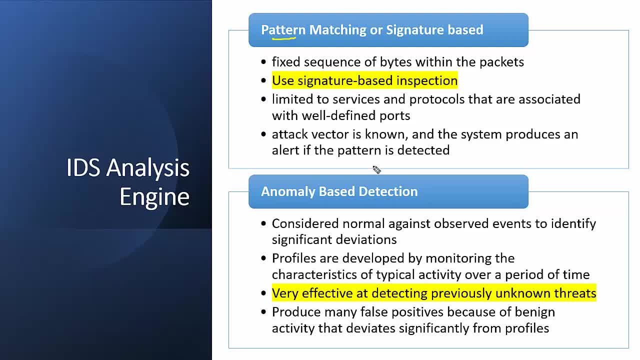 signature base. fast and very effective- you can say like that- but fail to detect the zero-day attacks on new attacks and all that. so pattern matching and signature base is basically use fixed sequence of bytes within the packet. it use signature based inspection limited to the service and protocol of layer 2. 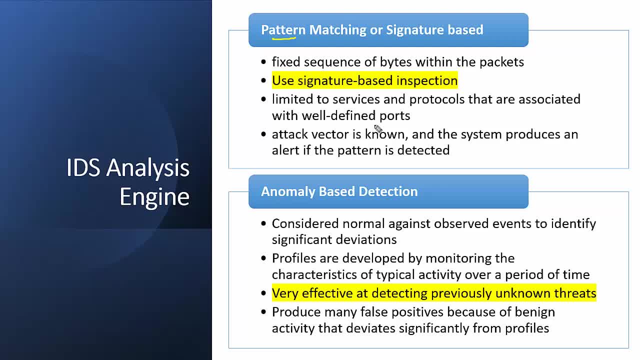 to layer 4: factors is known and system procedure and alert if the pattern is basically detected, which is mentioned here. example like this is the NIDS. we have just imagine okay and we have a web server here. example: this is my web server and we also have a attacker, so attacker basically send the packet. now this NIDS. 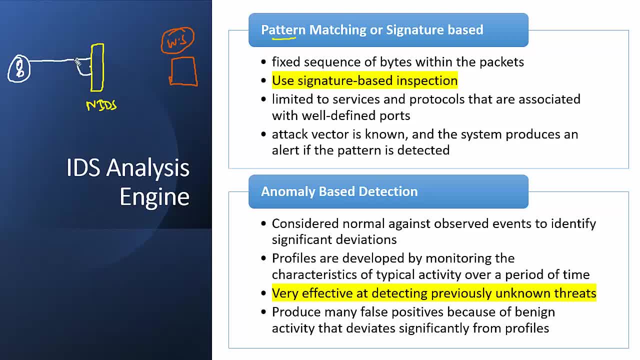 using a pattern matching with a pulse stopped element where this file is instant: seriae 12. link on the video site called N Silas. let me show you how to do. you can see the tie process actually here. this is the stressazon matches these codes for in data files we are always looking for potential of something. the resulting data-based. accurate because it's based on a very simple kolej action. so many will work, hoping you can imagine that. so it should be the purpose and you have this particular method in mind, to see something that means to lift up seeded data filesashi a pair of az and they just use three to range, and so I'm just going example here. so in the packet, the packet, what we have capture in cases that there is an element in the code of data fusion. so I've added the running date that's viewed in theDAOonent. 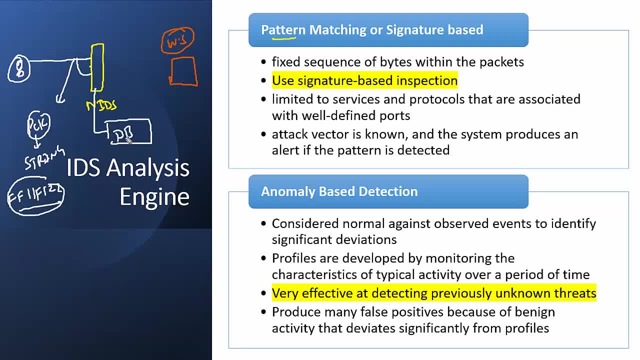 Then NIDS will check in his database and try to identify if we have any such kind of an attack with this kind of a pattern. If pattern match, NIDS will log the traffic. That is why it is called as a pattern matching signature base, or pattern matching or signature. 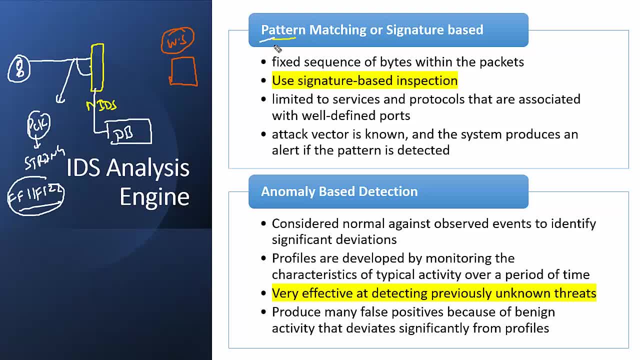 base intrusion detection. They check the signature, they check the string values in the packet and compare against the database they have. So that is how it works. But there is a one disadvantage of the pattern matching or signature base we have. If signature is not up to date with the new attacks or new signature is not there, then 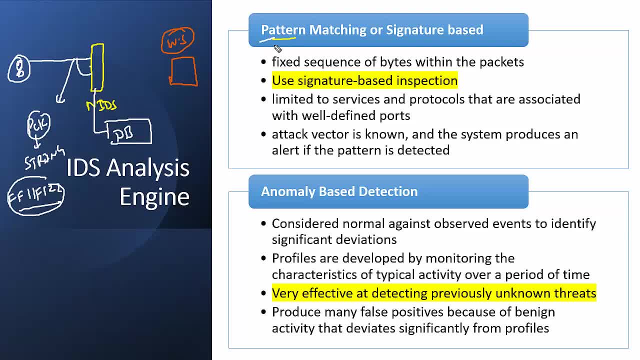 NIDS will fail to detect the new attacks. So that is the one concern we have: is pattern matching faster, effective, based on a signature base. In order to improve that process, we basically introduce the second one, which is called as an anomaly base detection, which is abnormal. 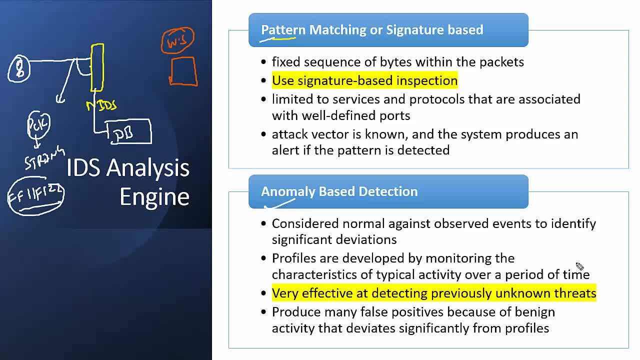 So in this case We basically what we did: we created a normal baseline and look for the deviation from the normal baseline. Example: source is any- sorry, like. source is any. destination is the web server. Source port is any. most of the traffic is coming on the port number 80 because we have 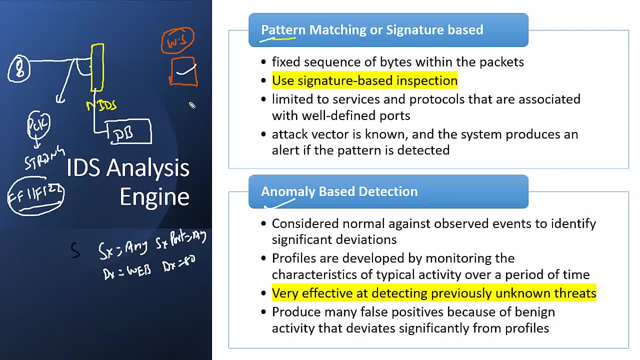 web server only Any traffic coming from outside it going on a port number 80. So we will look for any kind of abnormal behavior. If any packet is going against this traffic profile, I want that to be record because that is an anomaly. 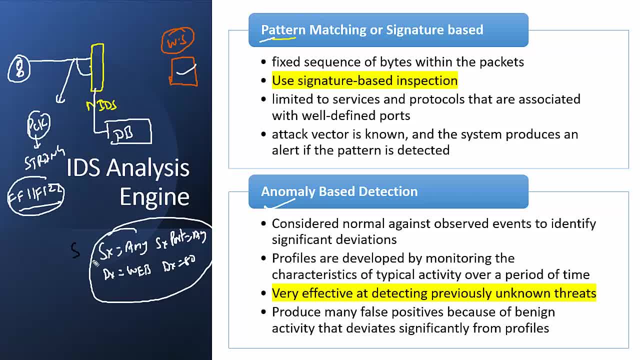 So we develop the profile initially when we install the solution. What it does it? it basically develop many behavioral attributes like number of emails sent by user, number of failed login attempts, number of host. number of packets are going on this port. 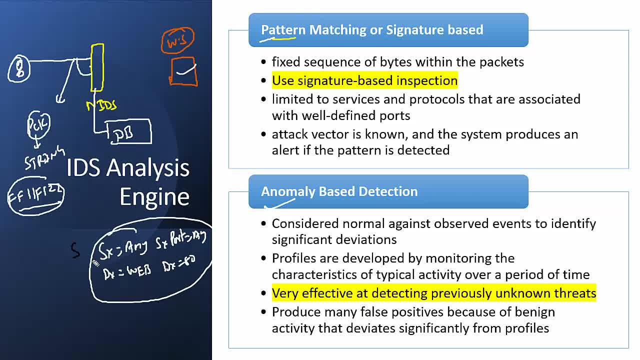 Tell net item by route user or tell net item by some other things. So this kind of a profile behavior we have created. So whenever such kind of a profiles comes to such kind of a traffic comes, we will basically compare against the traffic profiles. 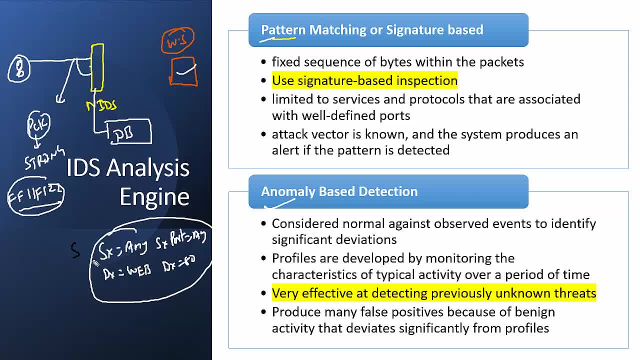 If it's basically going against that, it will record that as an intrusion Example, like for login attempt. it's a common thing. But if we discover more than 567, which is against the deviation, it will record that as an intrusion. 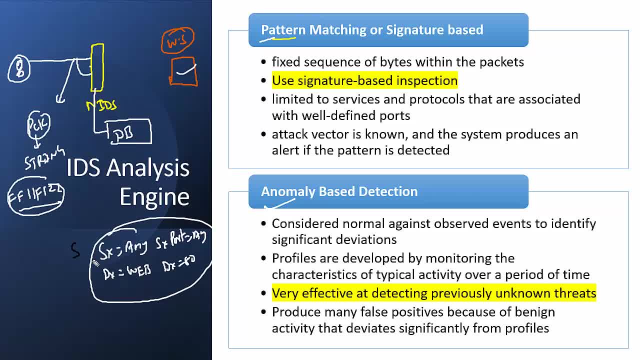 So, instead of checking based on a signature base and all that, They observe The behavior Of the traffic. Today we using the advanced version of anomaly, in which we introduce the AI and ML, which is called as a network behavior analysis anomaly, where we analyze the behavior apart from checking. 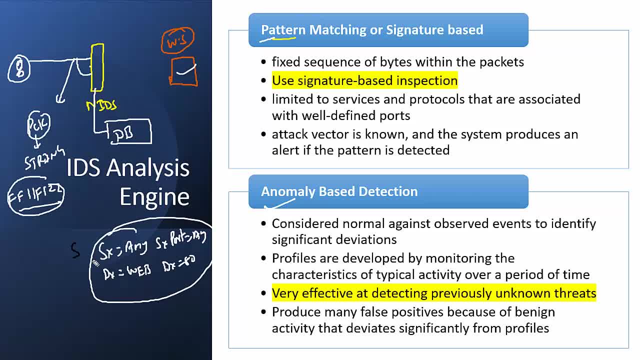 the signature and based on that, they record the intrusion. So it's very effective at detecting the previously unknown threats. because we have created a traffic profile for that. Okay, But it generate a lot of false positive traffic, Okay. So this is called a pattern matching or signature base or anomaly. 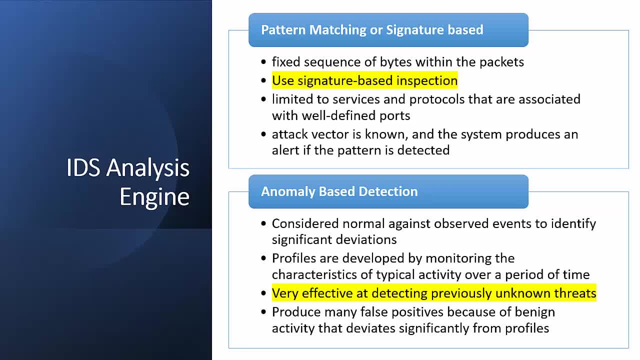 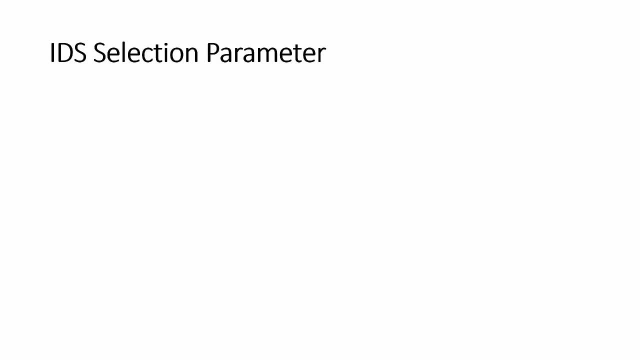 Anomaly based detection, which is also called as a network behavior analysis. Let's move to the next part. So we have discussed about different type of ideas. Then we discuss about the way to analyze the uh, the traffic intrusion, which is more like 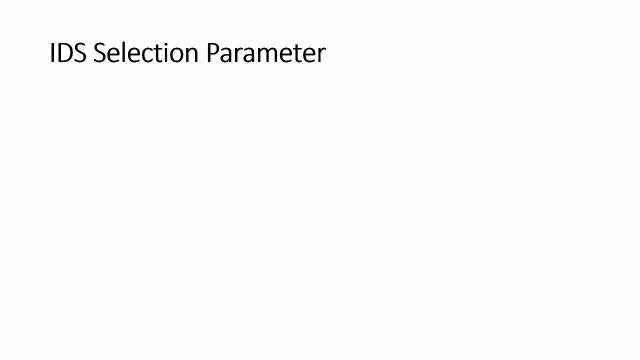 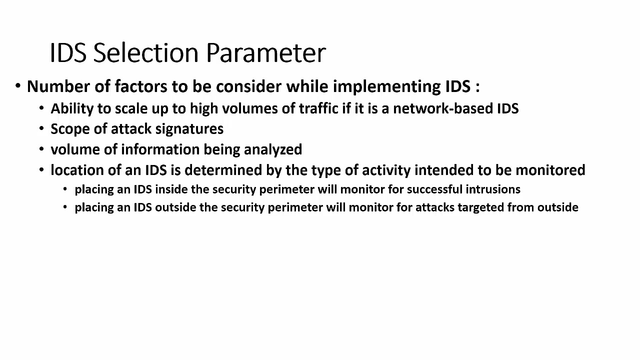 a base on a signature content based on the uh behavior. Now, when we implementing ideas in the organization, we consider several parameters. Okay, So we have a number of factors when you're implementing ideas. It's not something okay Randomly. we implement an IDS and HIDS. 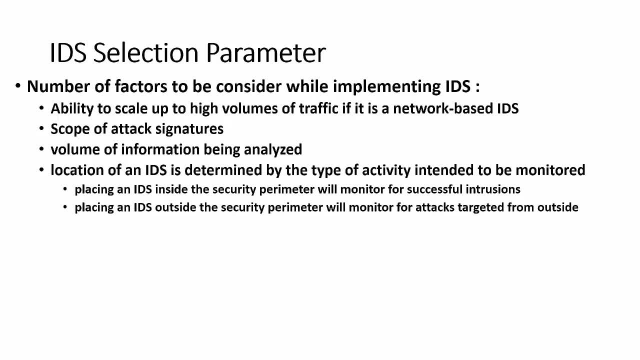 So we have a multiple parameters of: first is called about scale of traffic. If you know that, okay, we don't want a whole specific. we receiving more and more network traffic and all that. So, as a security architect, as a security consultant, as a security manager, we will. 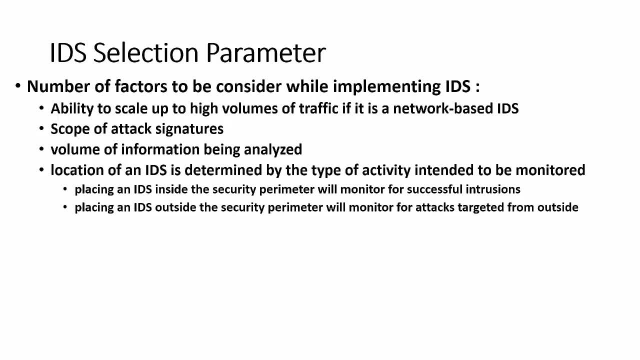 recommend to have a one common NIDS in the border of the network. So any traffic is coming from outside we can able to monitor. Now if NIDS I want to monitor for the internal traffic. So what is the best practices? 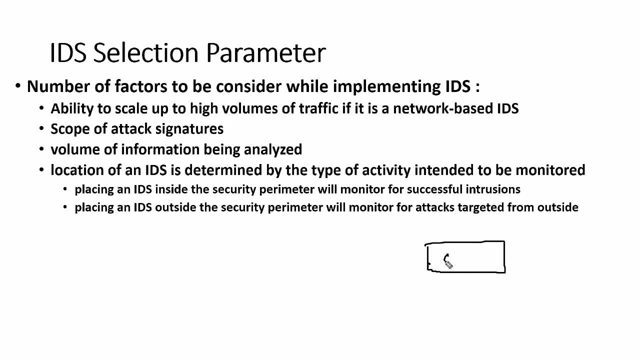 Um, this is my switch. Okay, As switch is basically work in a unicast- sorry, unicast- mode. So if we have a system a, we have a system B and we have a system C If a want to send. 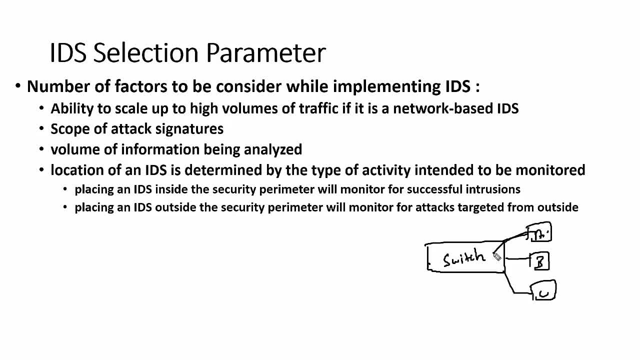 data to C. a send data to switch and switch will directly send the data to C because switch work in the unicast mode. But in that case, if I install the NIDS And NIDS want to capture the traffic stream and all that, it will not possible. 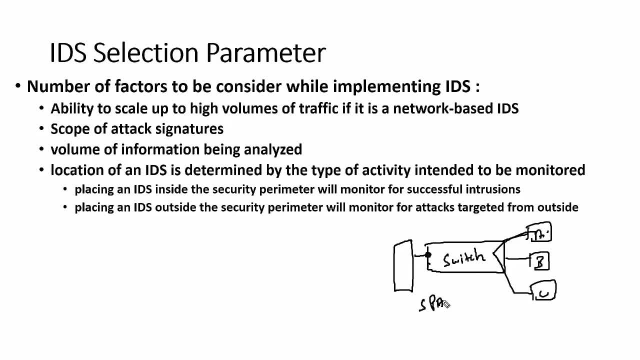 So we need to create a span port. We call it as a span port, mirror port, we called, And that port is basically mirror with all the ports. So if a sending any kind of a traffic to C, the traffic is going to this port only. 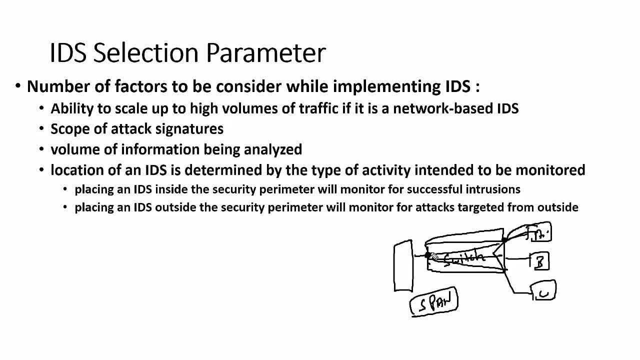 This port will send one copy of the traffic to this port. Make sure capability and capacity bandwidth of this port should be bigger than other, because that port is handling the copy of the traffic which is coming on these ports. Okay, So when you're planning for a you, you have us. you know you have a huge traffic network. 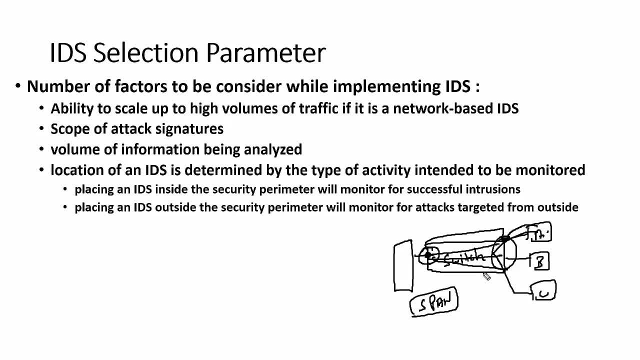 quantity and all that. So according to that, you can need to place the NIDS might be sometime. one NIDS will not be effective, So we installed the multiple NIDS which work in a fail safe mode. Okay, So if one NIDS is down from another NIDS, we can able to inspect the traffic. 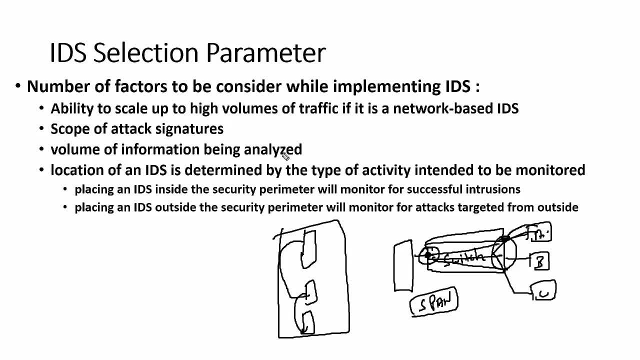 So this is how we can able to create the load balancer. Second is we need to improve and increase the attack signature, because that is the one concern with signature based IDS: It will fail to detect the new attacks. So on a regular basis, we need to update the attack signature so it can able to discover. 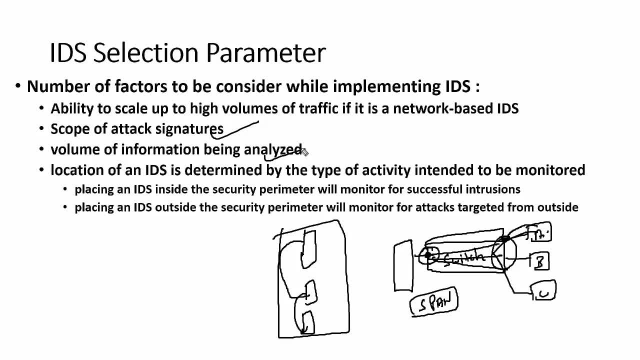 the new attacks. Third is we need to focus on the quality instead of quantity, because more data we collect, more time it'll take to do the analysis and all that. So it's it's very important during the anomaly, we create a more granular traffic profiles. 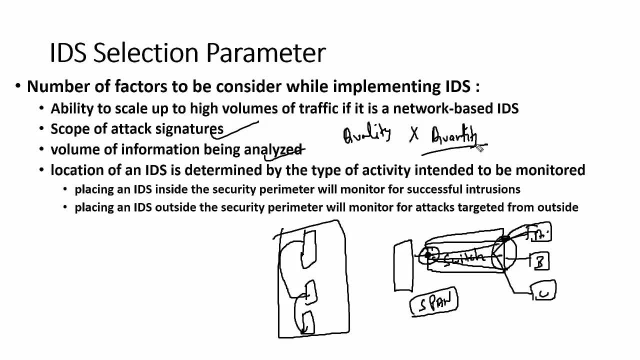 and that is only possible when you install the IDS. It will be in a learning mode where he will discover- or the tool is discovered, or device will discover- more and more traffic pattern. So that is another important thing: The placement of IDS. it's also play a very important role. 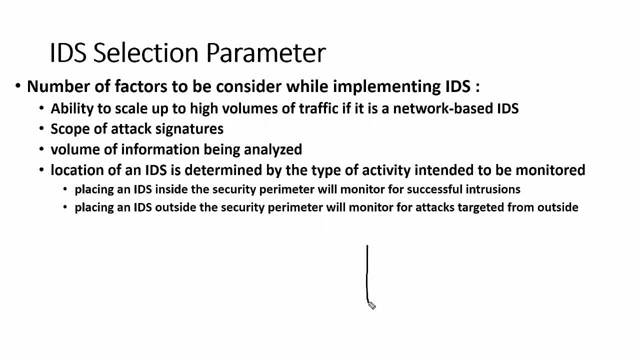 See, if you place the IDS inside the security parameter- example, this is the firewall we have- and then you basically install the IDS here, Okay. So, example like this is the IDS we have. Sorry, I'm sorry. So if you have an IDS here and this is the firewall, 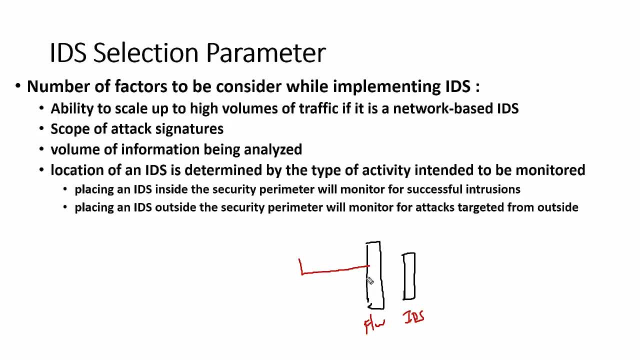 So traffic is already restrict the firewall, so firewall already filter the cream traffic. and then it, the cream traffic, is going to the IDS. Okay, so IDS will basically focus on the quality traffic, Okay, and anyone who tried to bypass the firewall and able to hack any servers or other servers. 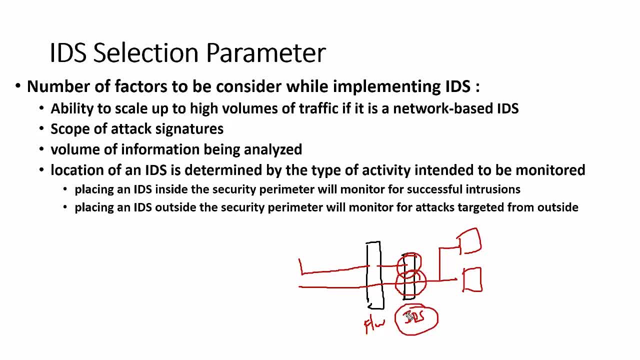 will be able to access the IDS. Okay, So if you place the IDS, if you place the IDS before firewall here, then what happened in that case? it will monitor all kind of a traffic and the unknown attack pattern which is coming from outside. 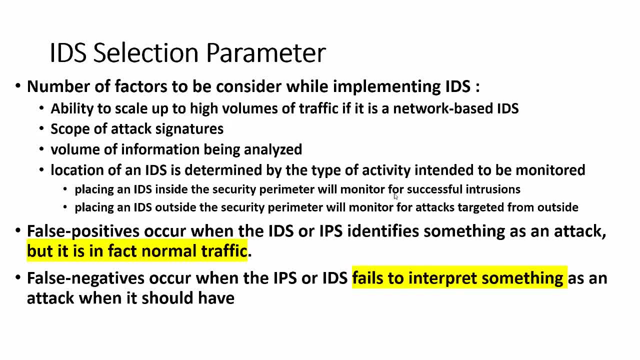 So, again, depending upon the business requirement, we can able to place the IDS. When you're dealing with the IDS, we have a two type of error: false positive and false negative. False Positive- So false negative- is when the IDS identify something as an attack, but in fact it's a. 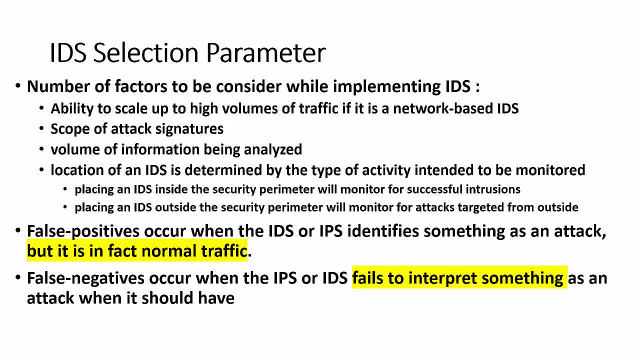 normal traffic. It will give alarm that, okay, someone has a password return, but in reality it is like a normal traffic. or there was a one day administrator trying to access from its home. IDS discover this as an intrusion, but in reality it is not an attack. 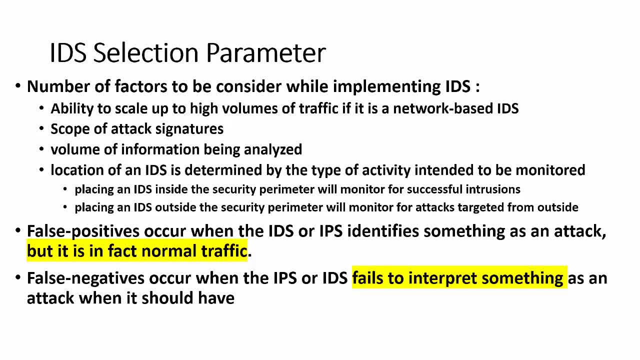 Okay, It's a normal traffic. So that is called as a false positive. Then second is basically called as a false negative where there was an actual an attack but IDS failed to detect. So for the any security consultant or any company concern is the false negative. 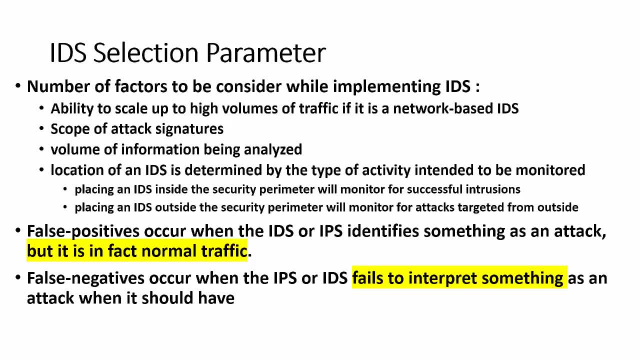 Where we have installed the hi-fi solutions and everything, but failed to detect the new intrusions and all that. Okay, That's why, when we're dealing with the IDS and IPS, we also have one more important metrics. One is called as a reporting and second is called as an event monitoring. 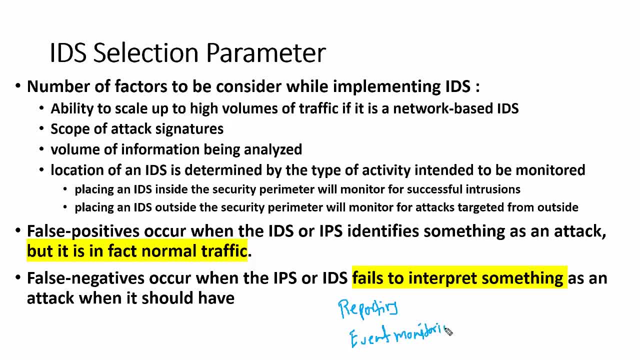 Now I've seen a lot of people get confused with these two words. Reporting is all about analysis based on the archive information. Okay, So reporting is all about analysis based on the archive information. even monitoring is all about real time monitoring. So IDS, what it does is it does an analysis based on the archive information, even monitoring. 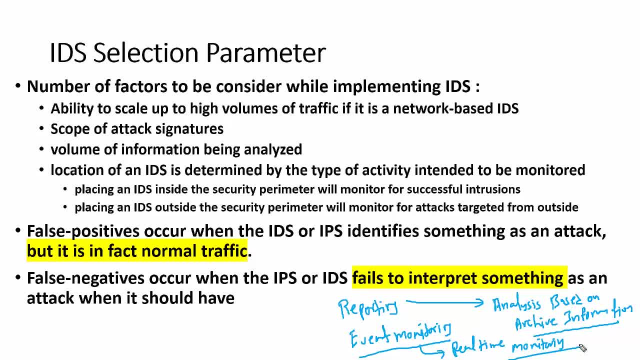 is all about real time monitoring. Okay, So what it does, it does first even monitoring and then it will basically document as a report. Okay, That's why, in order to remove, reduce this false positive and false negative, then we need to tune the sensor more effectively, tuned to ensure these are kept to be minimum. 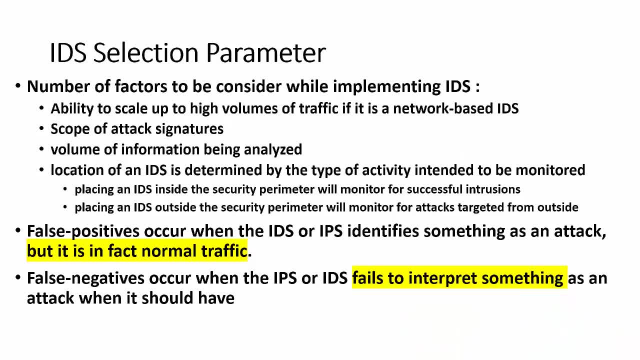 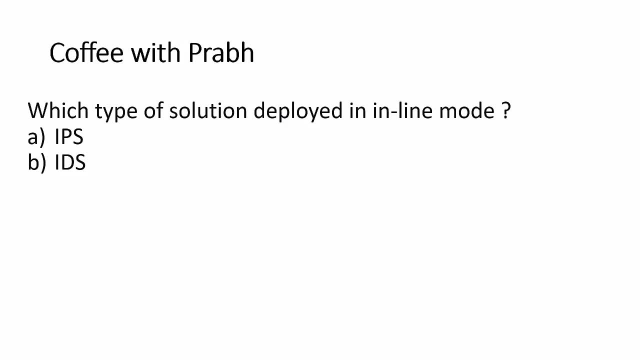 This false positive and false negative need to be keep minimum. Okay, So this is all from my side, So let's have some questions. Okay. So first question: which type of solution deployed in an inline mode? IDS is outline. We left with IPS. 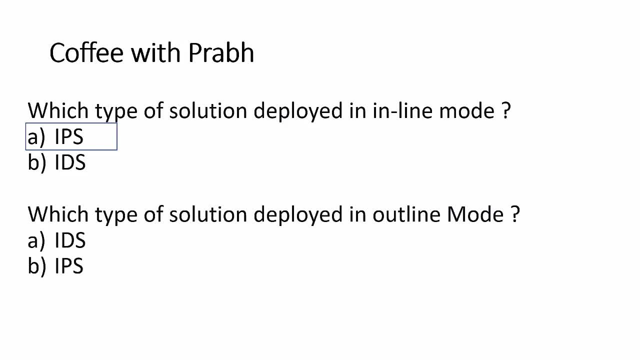 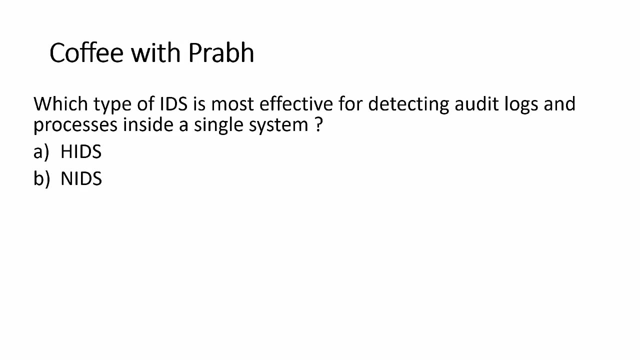 So answer is basically IPS. Let's discuss the second question: which type of solution deployed in an outline mode? Answer is IDS, which we have covered. Next question: which type of IDS is most effective for detecting audit logs processes inside a single system? 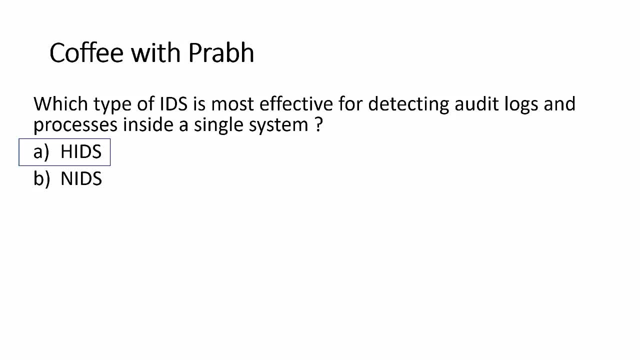 Keyword is single system. That's why I'm going with the answer. Which type of IDS focus on analysis of the network traffic? The answer is an IDS. So if you find this video useful and you want more content like that, do share your comments. 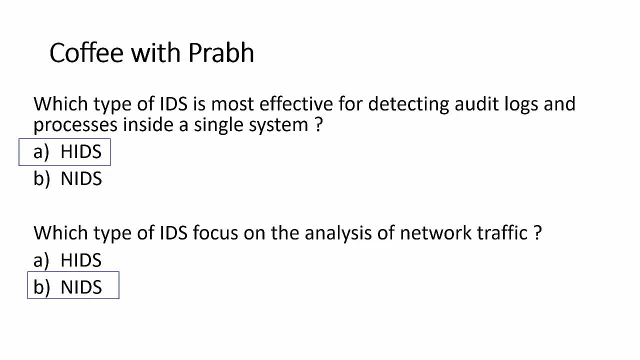 Do post your comments on the video, What kind of a video you want from me. from next time I will try my best to make a video and planning to make more contents, like in this format, where I cover the content along with that, Okay. 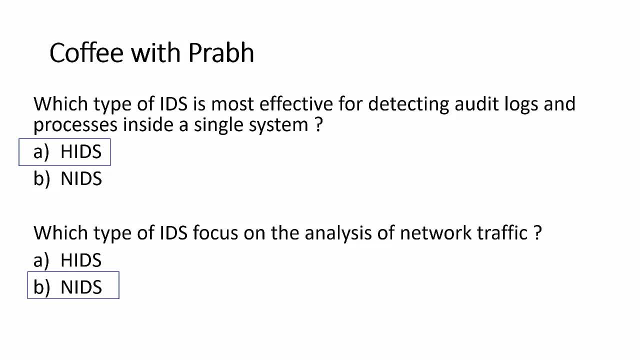 If you have any questions, please feel free to ask them in the comments below, And if you're new to my channel, do subscribe to my YouTube channel and click on the bell icon to make sure you should not miss my future videos. Thank you.